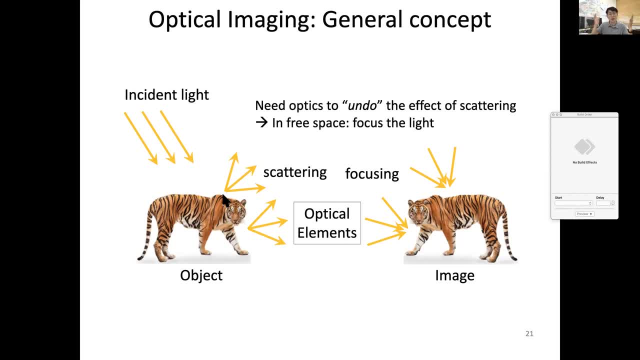 the light will interact and it is kept up. Remember, scattering is a photon and not only photon. kind of the particles deviate when it hits with an inhomogeneity. So there comes the scattering from one point And somehow, if those scattered light 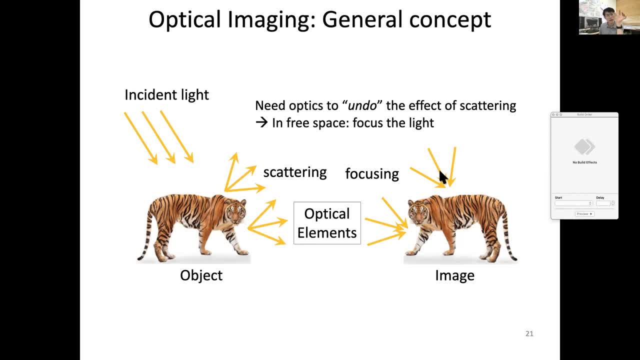 is in imaging space, if those scattered light will focus down to point, another point, which is a point point mapping in space. let's say, another point also focus down to another point corresponding. In this case it's kind of flipped, but let's assume that doesn't. 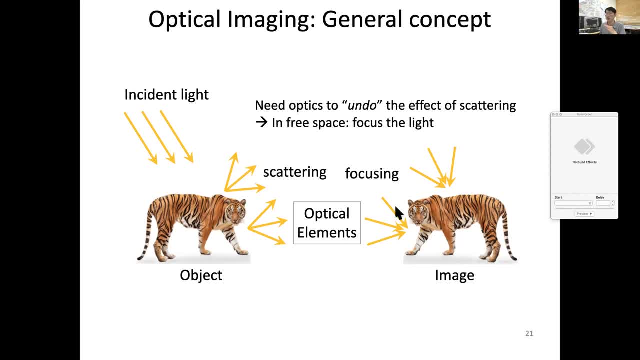 really matter, Then we can have one-to-one mapping and so that we can understand in imaging space what's actually seeing, what's out there in the object space. So this is concept of a imaging. Okay, So in fact, imaging is a scattering process. 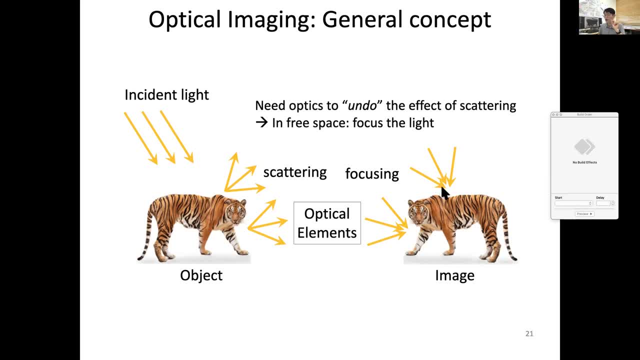 Has to be somehow to turn into a focusing process in a manner that you can have a spatial relationship. So for this, in optical imaging case, we do need some optics or optical elements to undo the effect of scattering, And in free space we should focus the light. 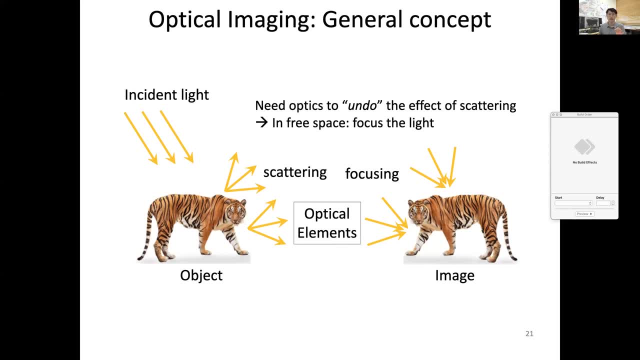 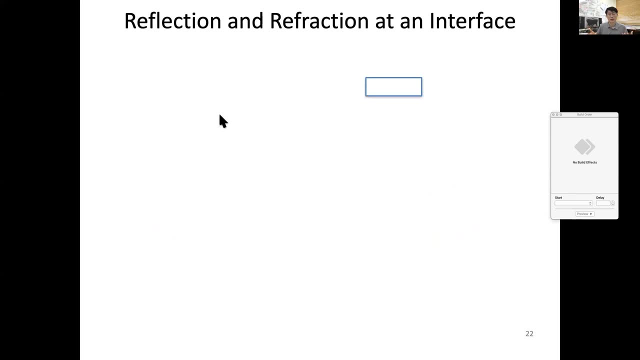 So this is concept of what we call as an imaging. For that we need to seek out what kind of optical element we can actually focus it down And also the property of the light interact with an optical element. So for that, the basic one is its reflection and refraction at an interface. when a wave 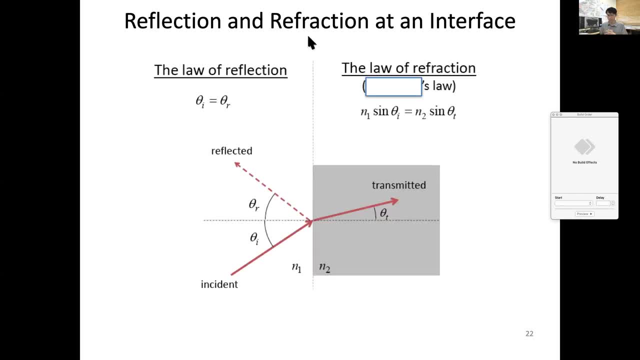 interact in this case Or, of course, light. So you already learned about this from previous years, So you already know about this from previous years, I believe. So there's an interface. We have reflective index of N1 entering into N2,. 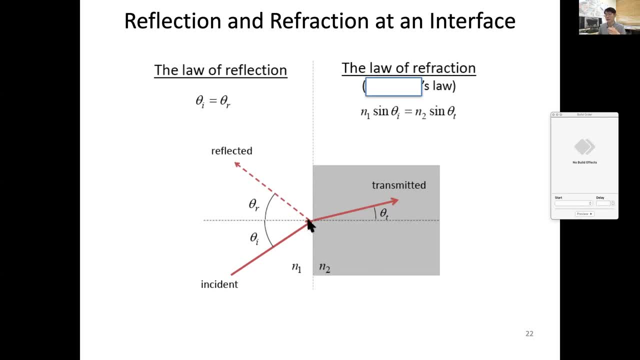 and let's assume we have instant slide, which is our leak angle, Then what can happen is, I said, at the interface, some will be reflected and some will be refracted and transmitted, but the angle will be changing. And if you think about the boundary condition of this electromagnetic wave, 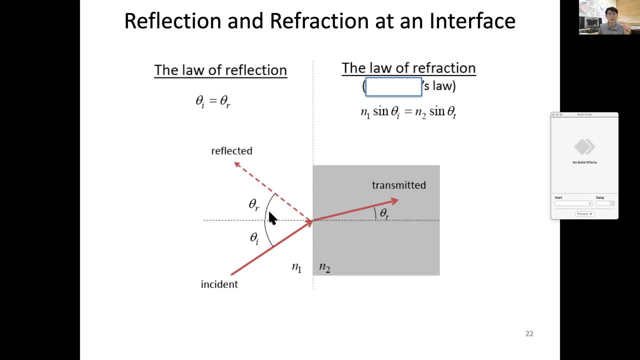 you will find out, the reflection angle will be the same. This is so-called famous law of reflection. What about the transmitted wave? So you can think of this as having N2.. Let's assume N2 is bigger than N1. What that means is the wave will slow down. So if we have a kind of a 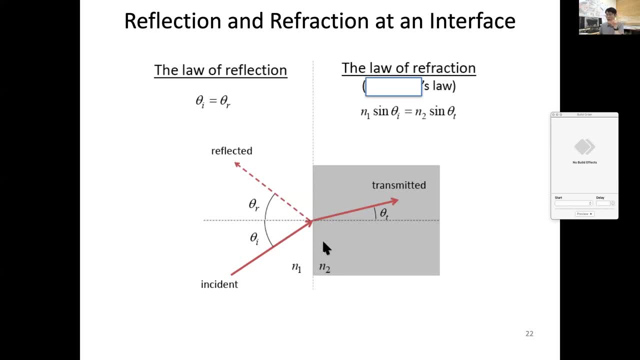 field, two two-wheel elements going in and this part will slow down, so the wheel will change this direction and going this way. So this phenomenon is a refraction and that relationship can be easily computed by calculating the speed of light change with respect to different. 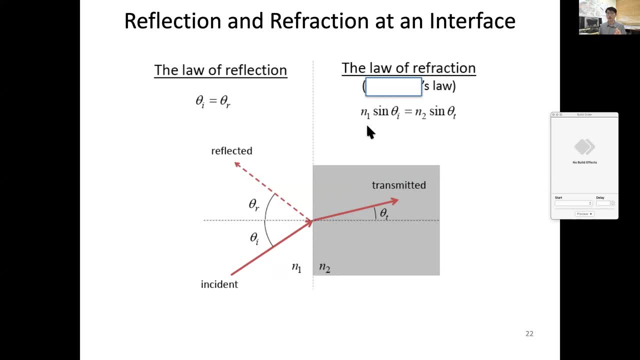 refractive index And that comes out turns out to be N times sine. theta has to be conserved. This is so famous that the law of refraction- and you already heard this- is so well known for the Snare's Law. So what it here means, like previous class time, as I said, 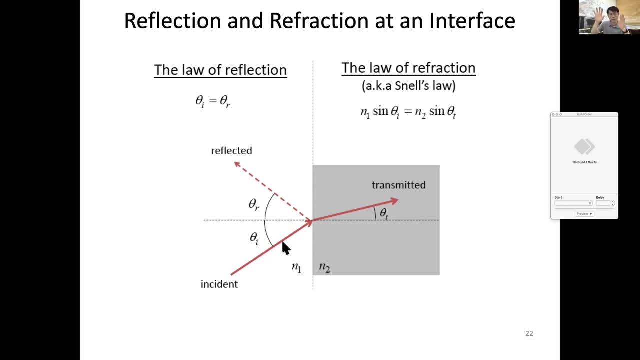 the waves tend to bend toward with higher refractive indexing index. Here you see the waves going and then in mid-term interface, because this is higher effect index, it bends towards the higher effect index And this can explain the mirage and moving effect. 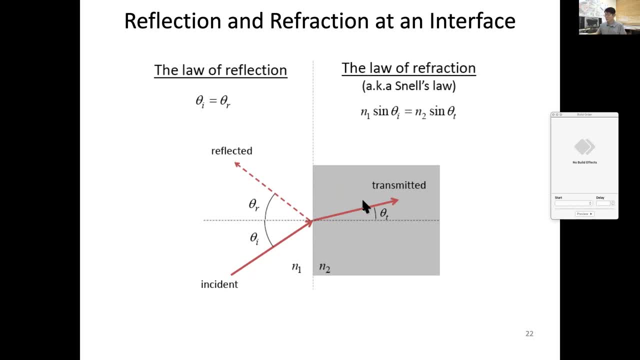 last time so that you can actually understand this. of course, there are other ways how to explain this. so, for example, let's say this is the, an ocean and this is a land. let's say there's a, a guy here, uh, watching if someone is uh, uh, swimming and try, uh and lost and dying. so how? 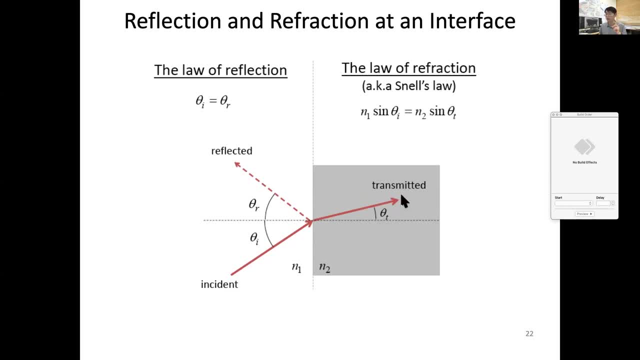 this guy will, um, will, go to this person to save him or her the way. uh, the problem is, this is an ocean, it's swimming speed it must be slower than running speed. then the guy has to find an optimal path to reach the minimizer time so that the speed of v1 and v2 are known and you 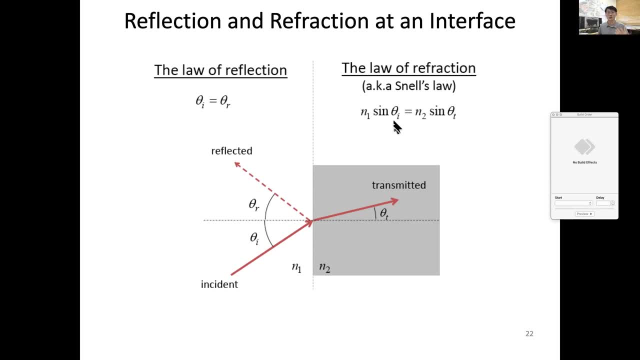 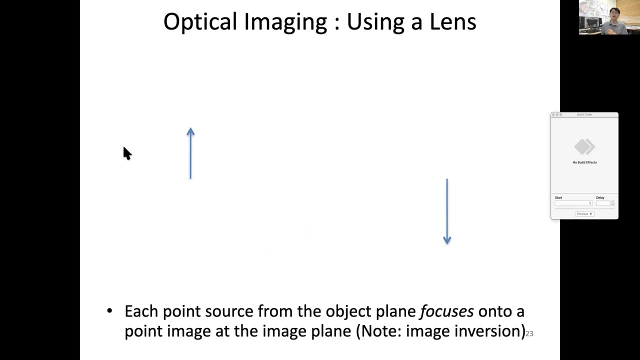 can find this path and that actually gives this interesting scenario. so this is a very interesting phenomenon if you think about this, how to derive this, and there is a very interesting ways of interpretation of this natural. now, the phenomenon i said about imaging is really an object has to be onto our retina so that we can make a sense of this imaging space. 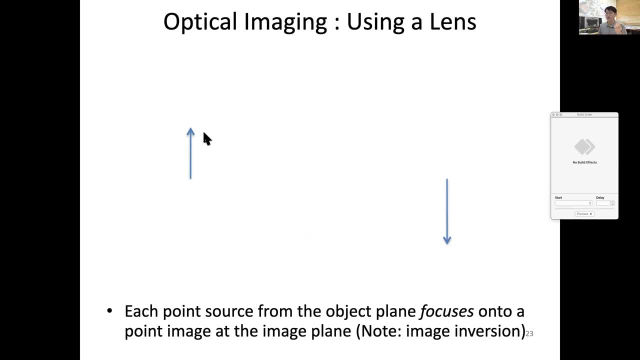 out of this object space. so we said the light has to scatter from a point and it has to focus to the point of this imaging space, so that this is kind of our eye. in fact we have a lens inside our eye. this is exactly how it works. so there is an object as a green light is. 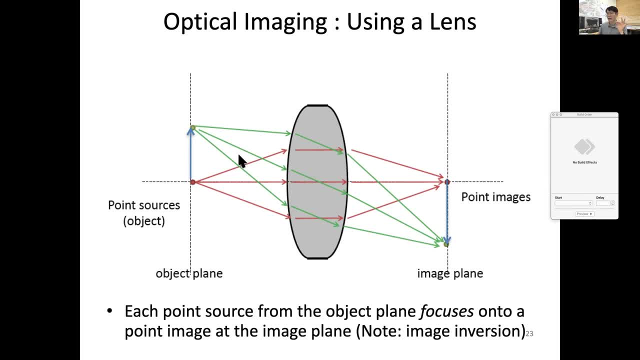 the light emitting from or scattered from this arrow head, and that has to be somehow converges, so diverging, And in fact, like the one I showed Snell's law previously. so this ray goes in and bend toward the higher refractive index. When it goes center, it doesn't change. 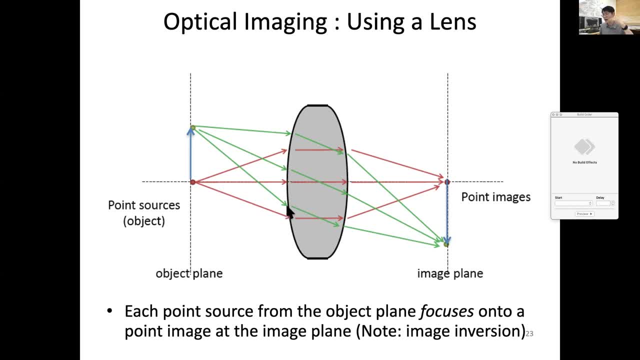 but it goes, this interface. it goes towards more higher refractive index. That eventually means the light somehow converges and focusing that, Likewise the rays, the light coming from the bottom of this arrow. some initially diverges, but through this lens 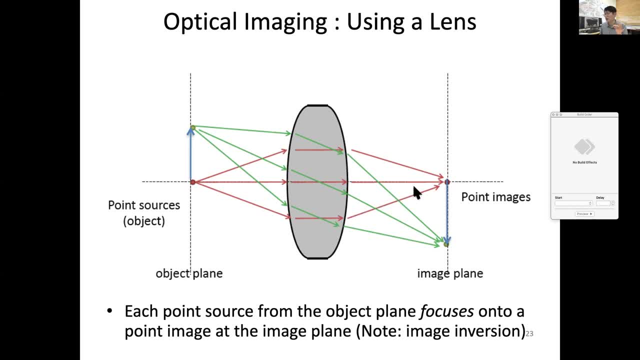 it bends towards this higher refractive index and likewise it will converge to a point. So it's a one-to-one mapping of this point images onto in the plane. So this explains what we are seeing and recognizing outside of the world. The light has to focus down onto our retina. 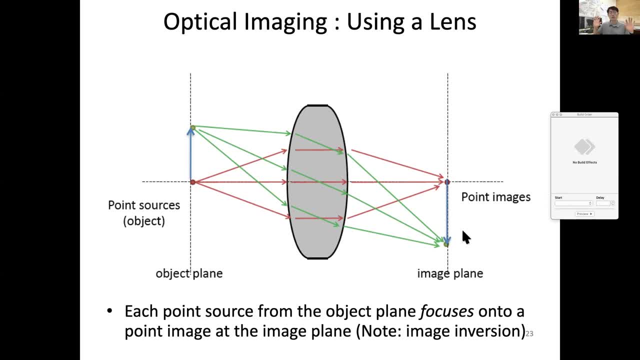 in a spatially consistent manner and one-to-one manner. Thank you.